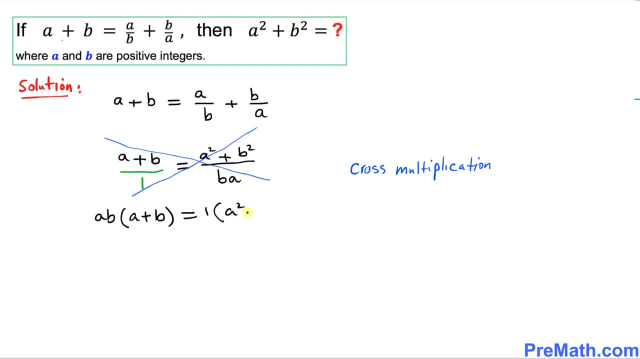 This is going to become one times a squared plus b squared. Now let's go ahead and distribute these. one. That is simply is going to become a squared b plus a b squared equal to this. When you multiply this thing, that's going to simply give us a squared plus b squared. 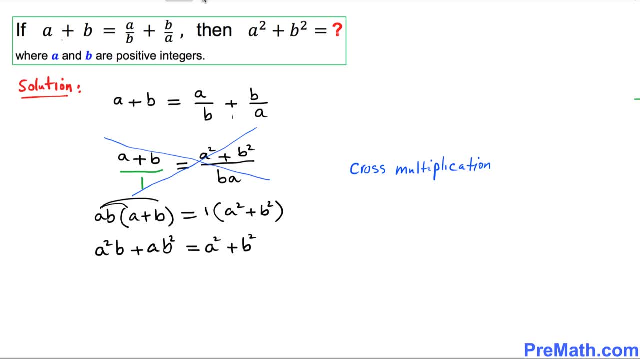 Now, in the next step, we are going to move this a squared And b squared on the left hand side. So we are going to end up with a squared b And if I move this a squared on this one, that is going to become negative a squared. 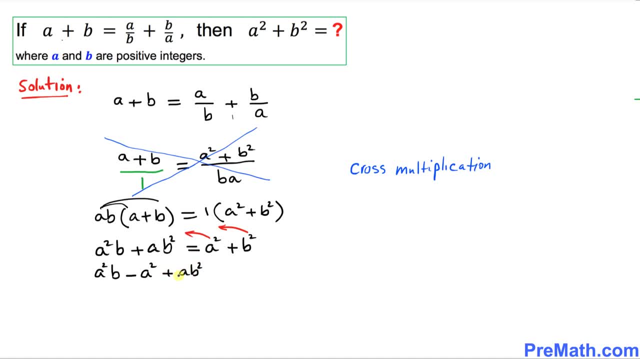 And then plus a b squared And then if I move this b squared on the other side, become negative b squared. So once again, This a squared, b is right here And a b squared right up here. And this a squared when you move it on this side, become negative a squared. 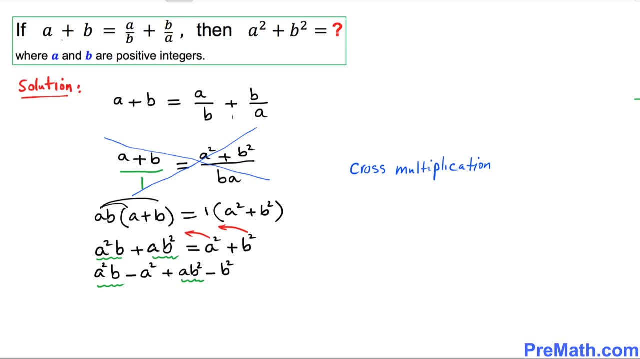 And this become negative b squared And simply we ended up with zero on the right hand side And in the first pair, as you can see, we can factor out a squared, So I can write down a squared times b minus 1.. 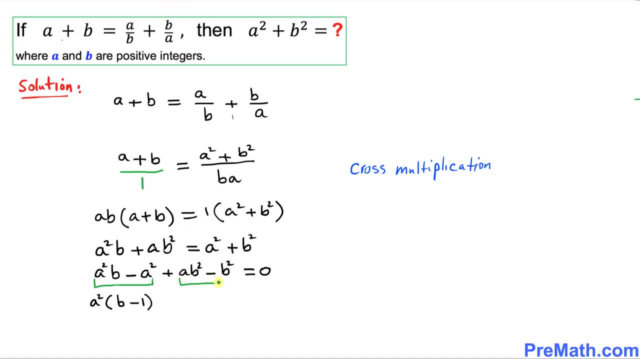 And likewise in the second pair right up here. we can factor out b squared plus b squared over here, And then times a minus 1, equal to zero. And now let's focus on this equation. This is the equation that we finally got. 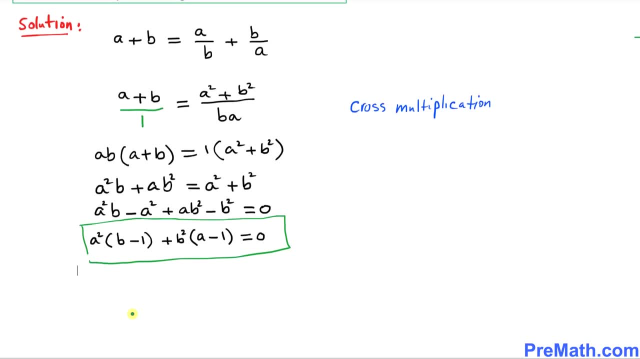 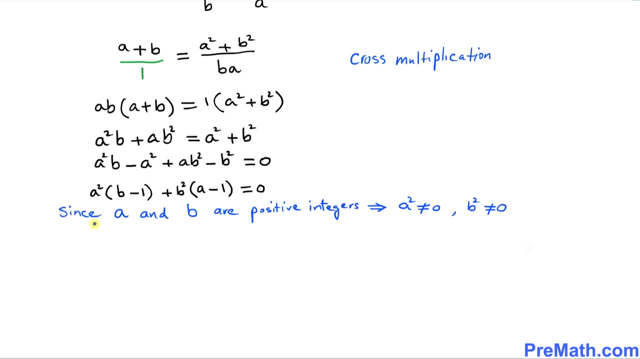 All right, We are going to take care of this one. Let me move this one a little bit up. And we know that a and b are positive integers. That means a squared cannot be equal to zero And b squared cannot be equal to zero.